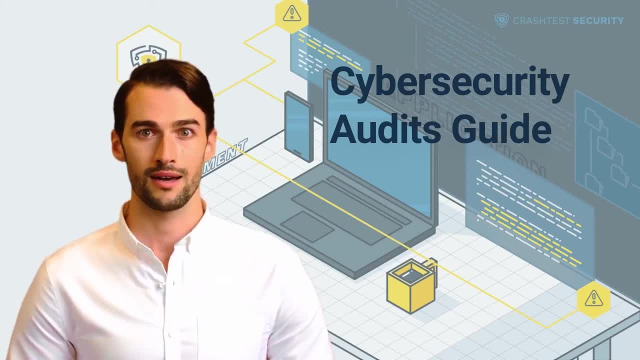 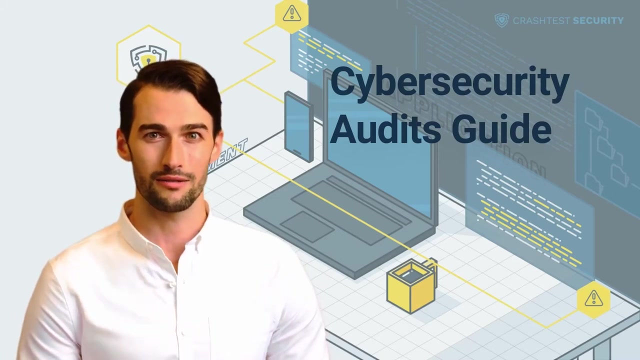 Hi, it's Alan from Crashtest Security. In this video, I will tell you more about the basics of a comprehensive security audit process, various aspects of an audit plan, audit types and best practices for continuous auditing. So let's get started. The modern cybersecurity landscape. 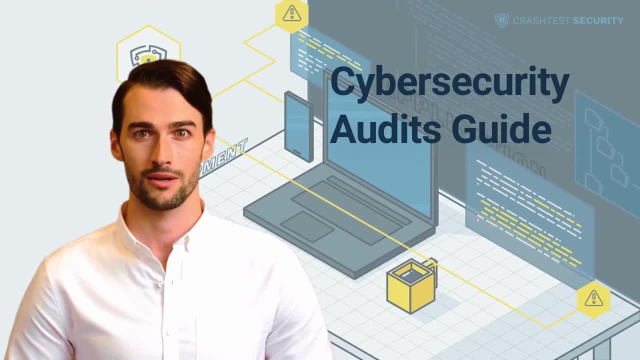 continues to evolve, with newer security threats emerging frequently and regulatory requirements changing to address them. As a result, tackling consistent threats is often considered one of the most effort-intensive tasks of an organization. This essentially starts with an organization's cybersecurity team assessing the effectiveness of existing security controls against emerging 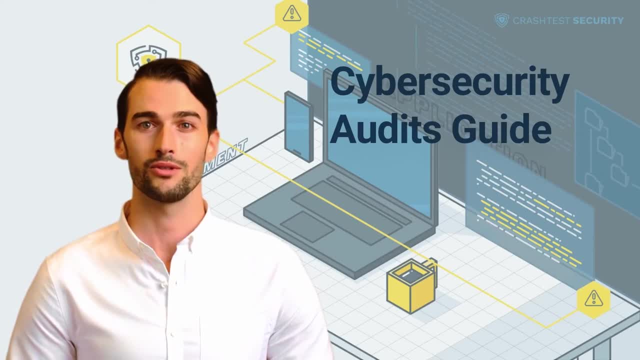 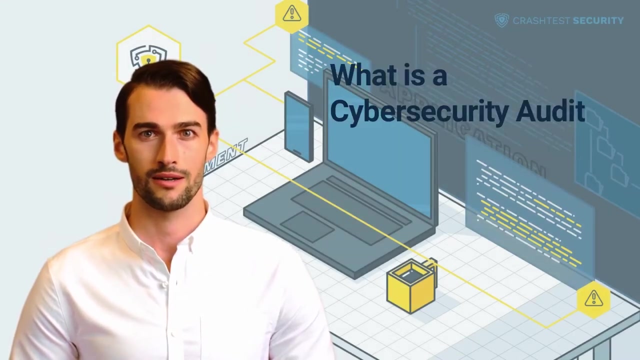 external and insider threats. To help with this, cybersecurity audits assess an enterprise system's security posture, including the levels of security risk, adherence to compliance regulations and the effectiveness of cybersecurity policies against potential threats. A cybersecurity audit provides a comprehensive assessment of the security and security requirements of an organization. This includes the level of security. 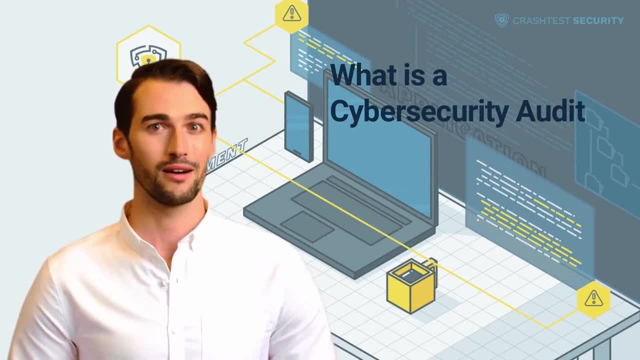 requirements of an organization, the level of security requirements of an organization and the level of information systems to evaluate compliance and identify gaps in security policy implementation. The auditing process involves closely examining the firm's digital assets and security controls to ensure they satisfy compliance standards requirements. Besides offering insights into 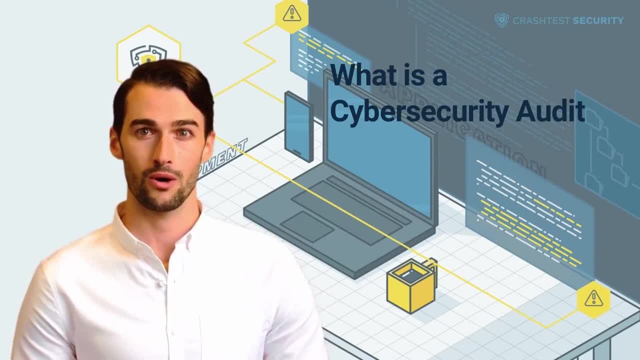 existing security vulnerabilities. a comprehensive audit also includes mitigation actions to mitigate cyber threats. An effective audit plan evaluates five core aspects of security Operations. encompasses the operations of an organization, the operations of an organization and the operations of an organization. A security audit analyzes operational framework, cybersecurity policies, security practices. 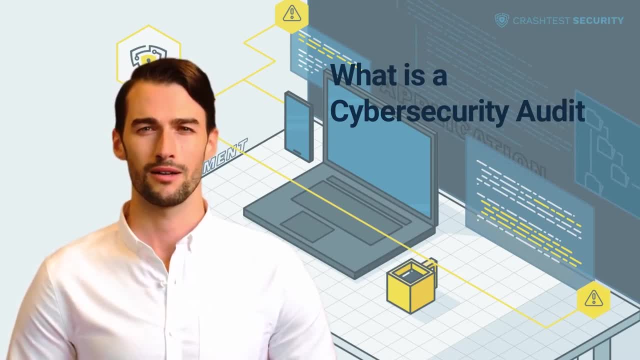 and controls. Operational security includes providing comprehensive safeguards on various infrastructure assets, procedural, functional and administrative functions. Network security security posture evaluation of network resources and other systems that can be accessed from the Internet. A thorough network security audit analyzes network availability. 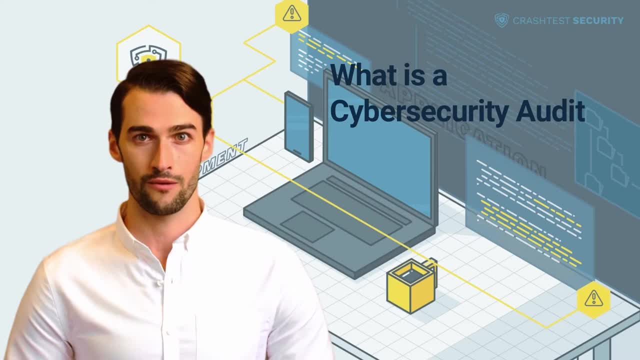 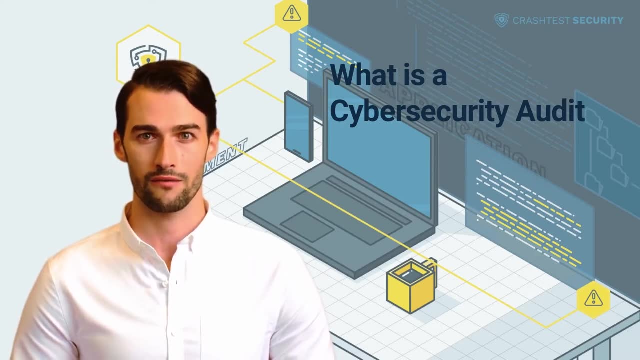 device access control, infrastructure security and the overall performance of network assets. Data encompasses the security measures and tools involved in protecting the confidentiality, integrity and authenticity of data within the business network. Data security typically includes TLS, encryption, authentication and authorization controls and security practices used to protect. 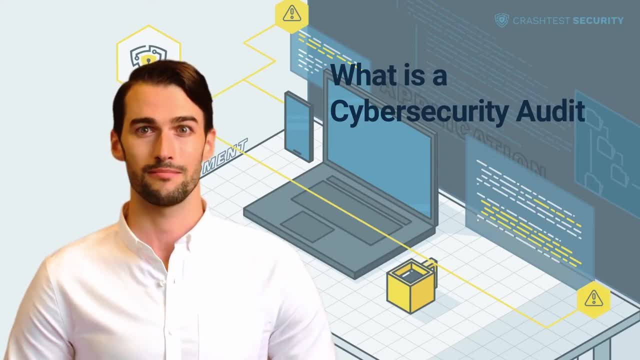 critical business data in transit and at rest. System refers to the level of security implementation in hardware assets, operating systems and other critical infrastructure within the network. System refers to the level of security implementation in hardware assets, operating systems and other critical infrastructure within the network. 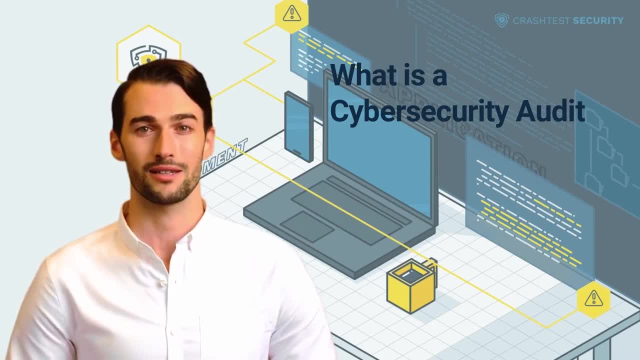 System security audits review the patching process, device access management and the management of elevated permissions. Physical security preventive actions and controls put in place to govern access to application data, software and hardware assets. Physical security measures also protect enterprise personnel from potential threats. 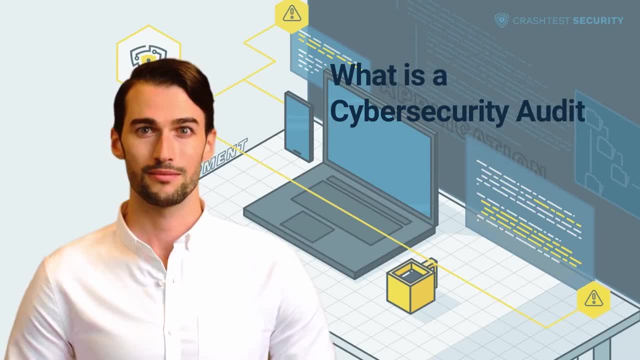 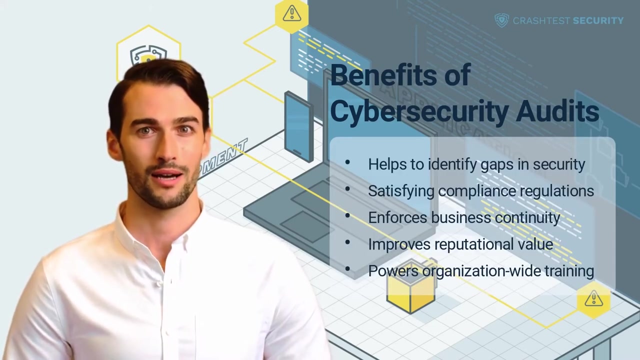 that could result in loss or compromise of business systems. Comprehensive cybersecurity audits evaluate multiple aspects of physical security, including surveillance procedures, access control and physical disk backups. An effective cybersecurity audit program helps evaluate and improve the security of enterprise systems, networks, connected devices and 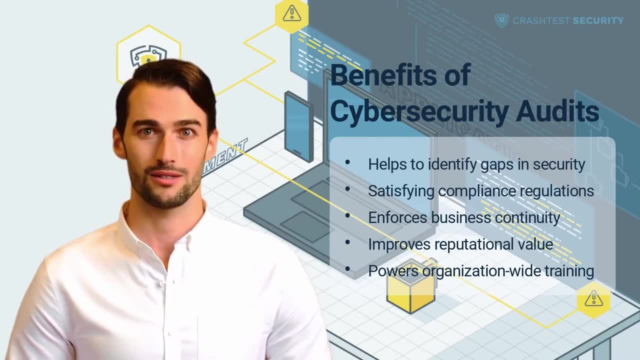 underlying data. Some benefits of performing a comprehensive audit process include the following: Helps to identify gaps in security. During a cybersecurity audit, security experts probe business systems for potential risks that can lead to breaches and disruptions. The auditing process includes continuously monitoring the entire business network to detect and identify flaws. 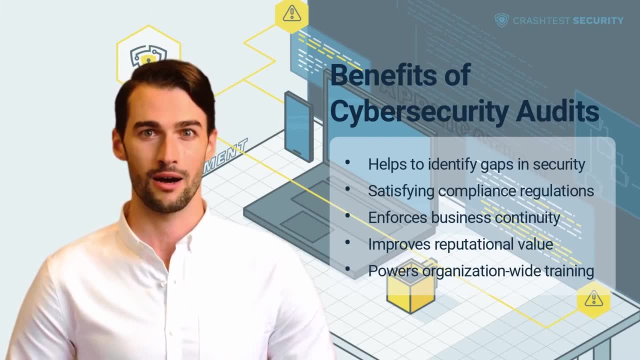 that can be exploited for an attack. Exposing weaknesses and high-risk policies helps security analysts create risk management plans and improvise an existing cybersecurity strategy Satisfying compliance regulations. All enterprise systems that process information are guided by security compliance frameworks and governance institutes such as the National Institute of 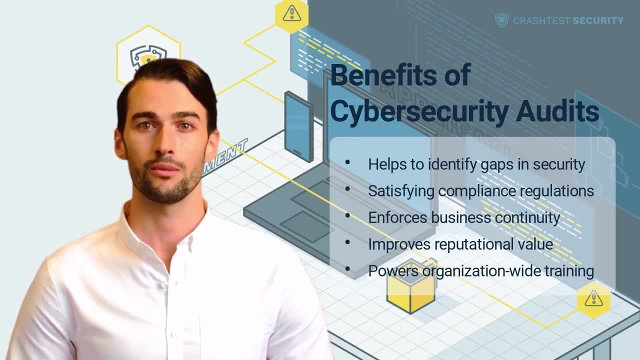 Standards and Technology, The Health Insurance Portability and Accountability Act and Control Objectives for Information and Related Technology. Such frameworks outline compliance audits as a statutory requirement, which help reduces the company's legal risk. Compliance audits determine whether the organization adheres to these frameworks' policies, rules and guidelines Enforces. 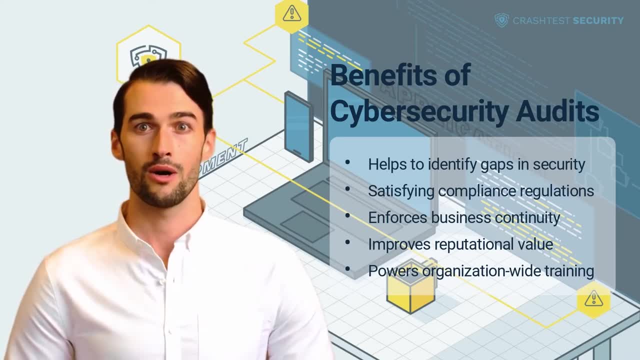 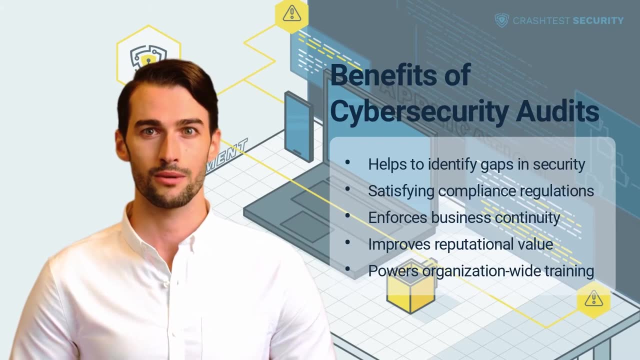 business continuity. A comprehensive cybersecurity audit helps identify security gaps that can be exploited to orchestrate attacks and document possible mitigations for an exploit. Security professionals and operators rely on audit analytics to administer appropriate security mechanisms for regaining control of key infrastructure already compromised by malicious. 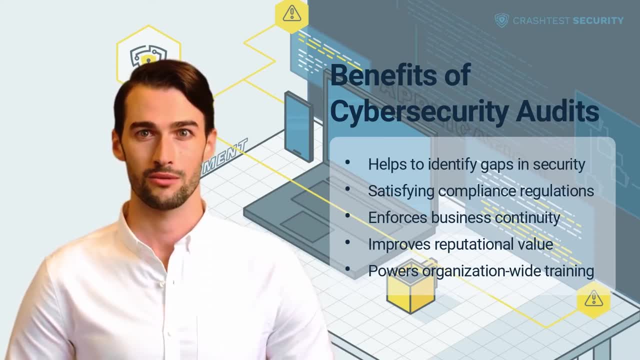 actors. A security audit includes backup and disaster recovery plans to ensure business systems are available during a security breach. The process ensures minimal business disruptions, even in an active attack. Improves reputational value. Cybersecurity issues damage an organization's reputation, since users avoid trusting a company. 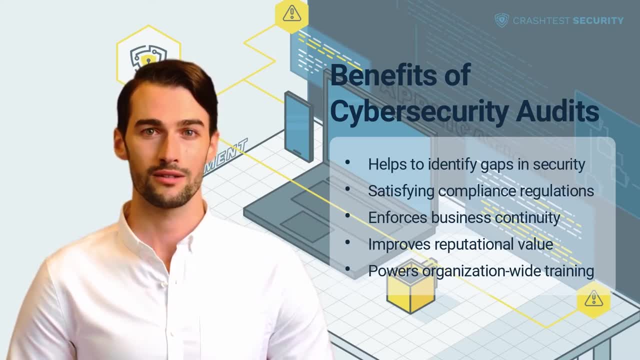 if it can't secure its digital assets. When attackers obtain user accounts or organizational data, they can access sensitive information and key infrastructure, leading to data breaches, application availability and intellectual property theft. Through regular audits, organizations can proactively identify and fix cybersecurity. 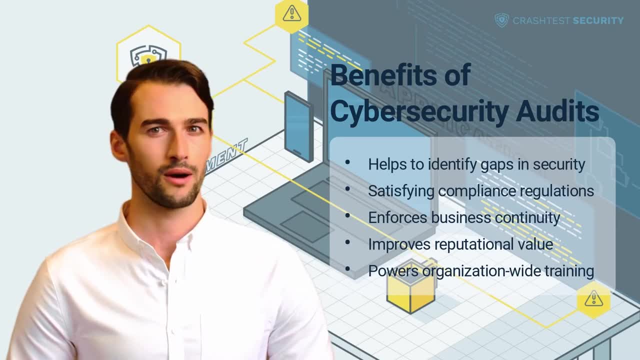 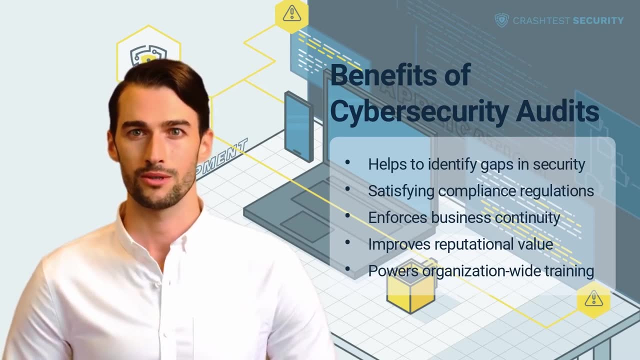 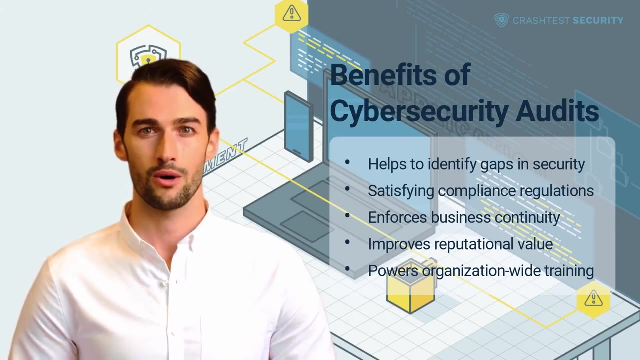 threats in the business network, earning public trust. Compliance audits also evaluate how the firm adheres to regulatory requirements and security standards, featuring the company's performance within its industry Powers, organization-wide training and cybersecurity awareness. A comprehensive audit includes a catalog of the enterprise's software. 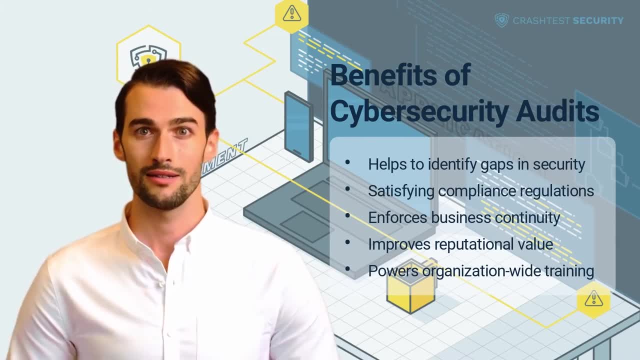 and hardware assets. The inventory consists of documentation of the security posture and potential risks of all components used within the business network, enabling everyone to envisage the organization's security threats. Audits also provide security experts with the tools and knowledge needed to improve the organization's cybersecurity. 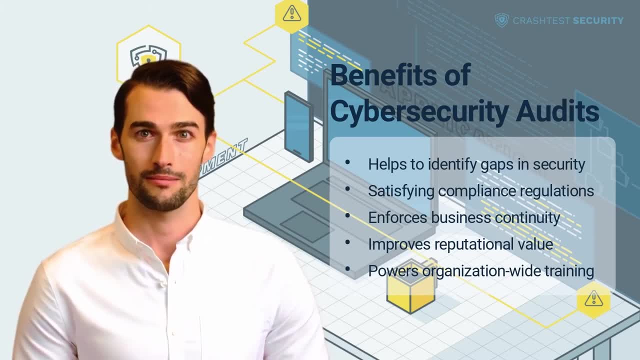 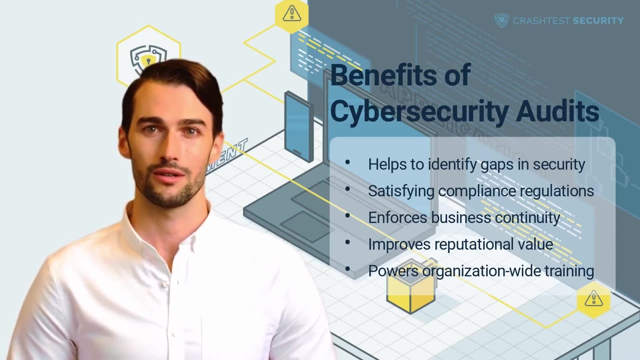 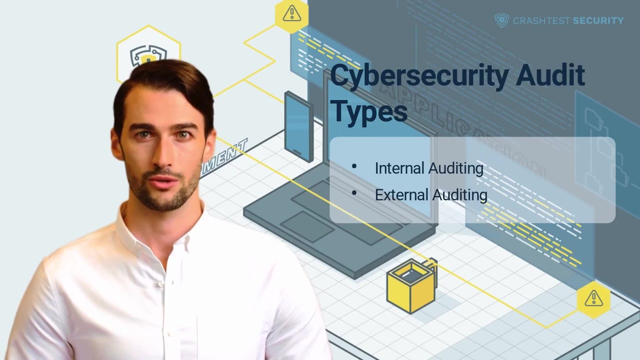 framework. In addition, the audit process provides a complete picture of the firm's IT infrastructure and an in-depth look into business operations, allowing the cybersecurity team to optimize security controls for safeguarding business systems. Audits in cybersecurity are categorized into Internal auditing. The in-house team performs 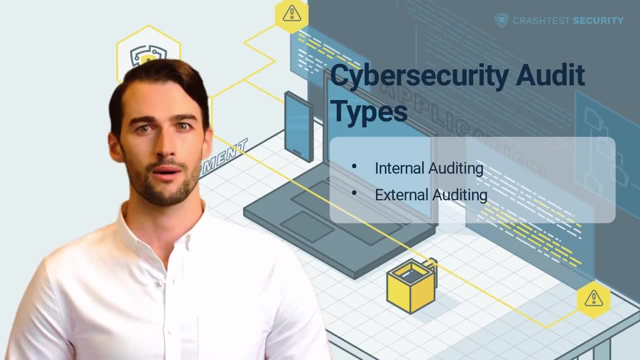 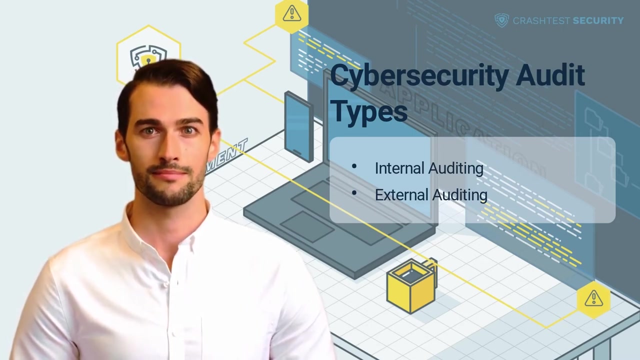 internal audits to evaluate the network's internal controls policies and cybersecurity processes. A robust internal audit foundation helps assess existing and required security measures, while assisting the cybersecurity audit team in understanding flaws in security implementation. Benefits of performing internal audits include Cost-friendly security evaluation. 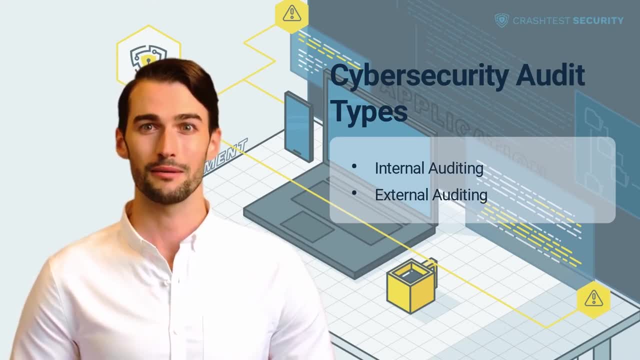 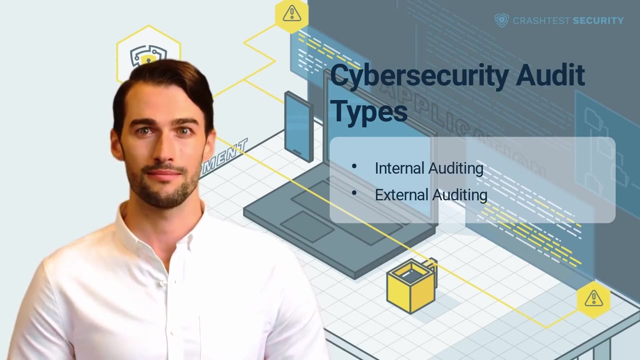 Offers more control over the auditing process. It can be customized to suit security systems in use. External auditing: In an external audit, third-party security experts examine security controls, regulatory compliance and security gaps within an enterprise network. External auditors are highly trained and qualified in identifying. 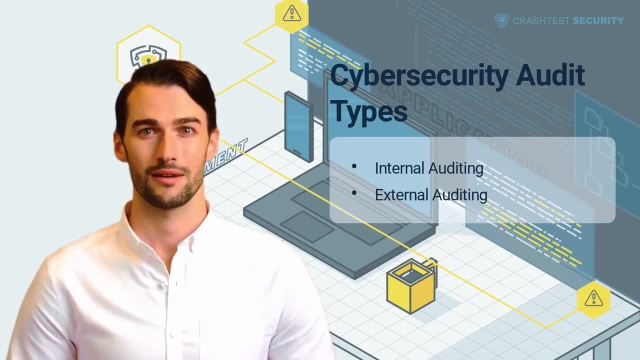 vulnerabilities, sensitive data and network assets. They ensure the auditing process meets the organization's objective by helping counter continuously changing threats. Benefits of external auditing include: Unbiased, experienced auditors with certifications and formal training. More efficient, since specialized security experts perform it. 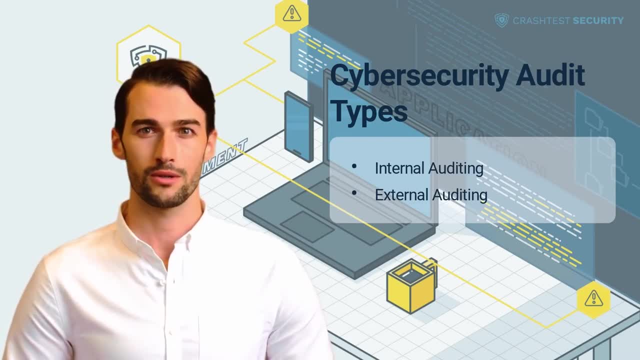 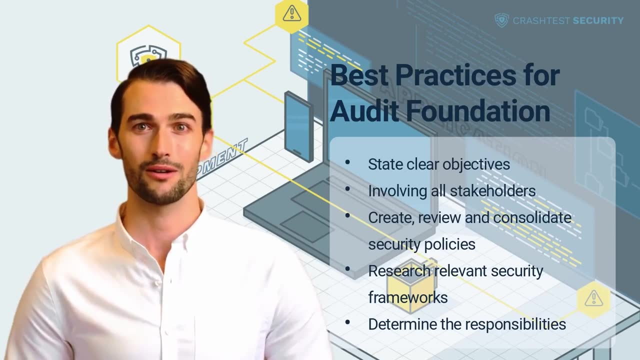 Ensures complete adherence to regulatory and compliance frameworks. A well-executed cybersecurity audit helps secured assets while offering guidelines for managing security risks. Some recommended practices to ensure effective audit processes include: State clear objectives. The audit team and security staff should start by defining the scope of the audit. This ensures the unambiguous identification of audit goals. 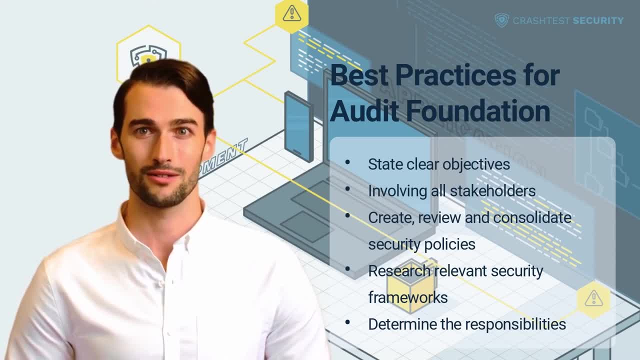 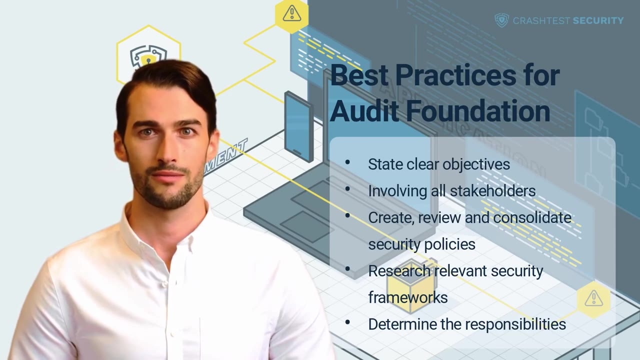 and the business objectives they aim to support. Defined goals and objectives also enable cross-functional teams to administer the audit process seamlessly without impacting the performance and availability of business systems, Involving all stakeholders- Every security staff, member, developer and non-technical employee. 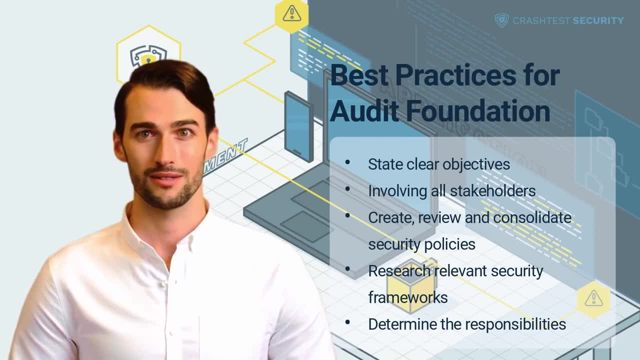 should know about the cybersecurity program and how it affects business activities. All concerned- business units and external vendors- should also be updated on the existing cybersecurity policies and their roles in maintaining the organization's security. The audit team must be able to understand the security posture With every stakeholder. 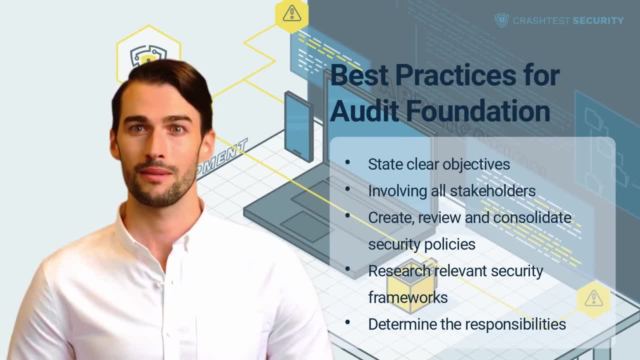 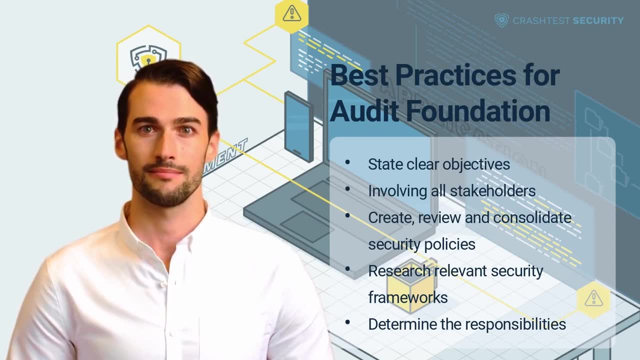 understanding their role in an upcoming audit, it is easier to conveniently plan the time, money and other resources needed to perform the audit. Create, review and consolidate security policies. Security policies govern how data is processed, stored and transmitted by an organization's business systems. Creating a security policy. 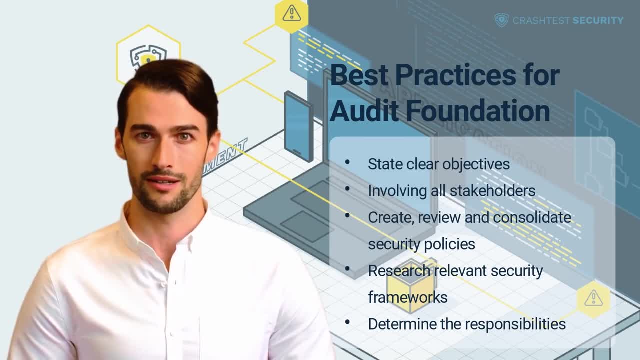 helps the audit team analyze how sensitive digital assets are and what security controls are required. for a more straightforward auditing process, The security policies should be stored in a centralized and searchable database, giving auditors a complete picture of the network's security posture without navigating complex workflows. Research: relevant security frameworks. 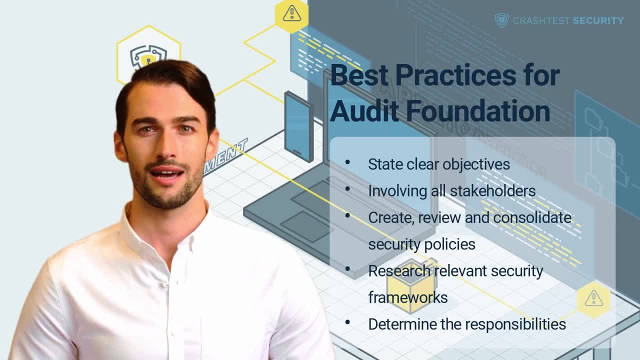 Each industry has different compliance standards that govern the storage and handling of sensitive user data. Security experts should determine the relevant compliance framework that encompasses a specific industry department to adopt only relevant data protection laws. The audit team should refer to specific requirements for each identified framework and outline the security.